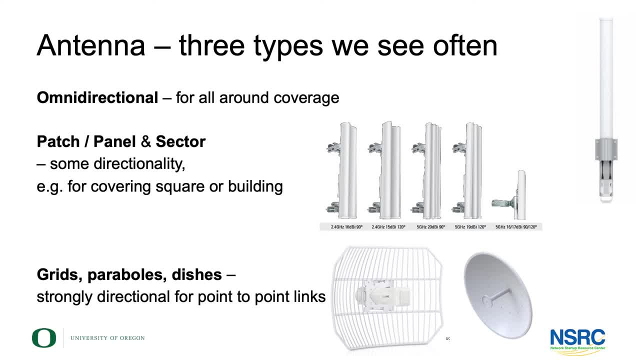 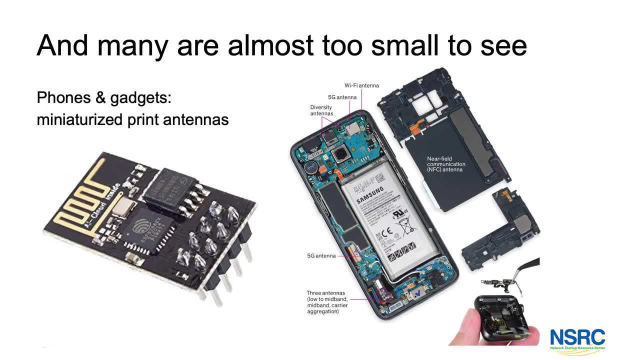 opening beam width, but they're quite directed. It's almost it's like a torch that you direct in one particular direction. Then there's antennas that are so small that we can barely see them. They're built into stuff, They're print antennas On the left. here you see. 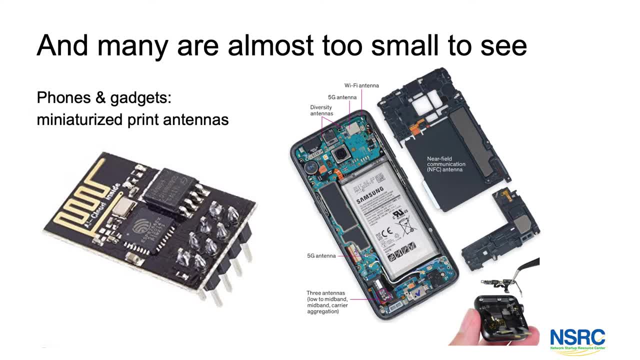 this typical meandering like winding river print, That's a Wi-Fi print antenna on a very small IOT device. here, Same in mobile phones- There isn't a lot of space and you have to fit in a lot of antennas- Wi-Fi, cellular antennas, Bluetooth- So they're printed antennas- very small. We typically don't see them. 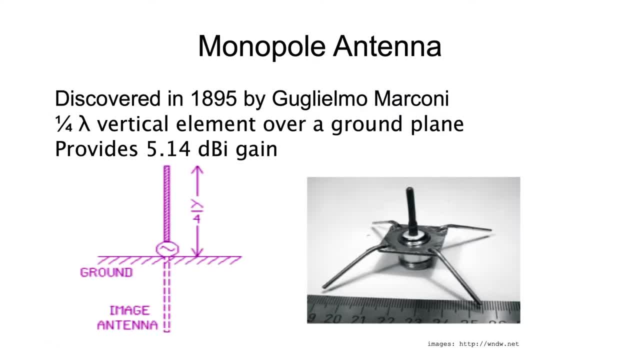 Here's another popular simple antenna. It's a monopole antenna. It's just a quarter wavelength piece of wire with four counterparts and the ground plane described many, many years ago, 125 years ago, and it gives us a gain of five dbi theoretically when we build it properly. 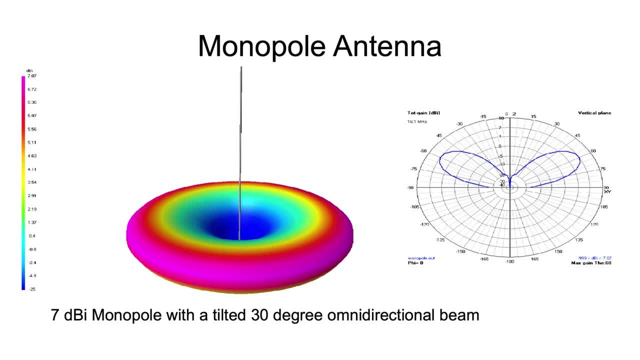 The monopole antenna, and this is an omnidirectional antenna. Seen from the top, it would be a circle. Seen from the side, and here, in this 3D view, we often say: it's a donut, If a donut is something you're eating. 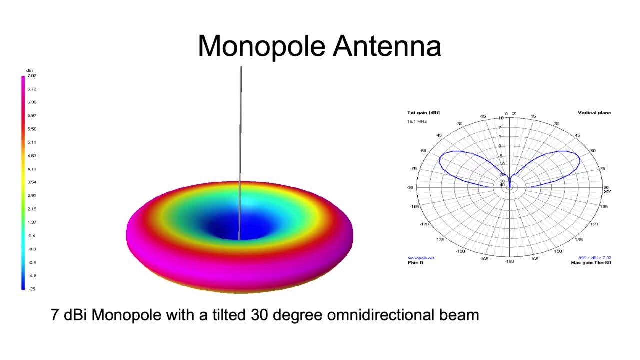 well, you'll recognize the donut structure here. Seen from the side, there is distinct directions in which it sends its power. Seen from the top, it's a circle. Note that it sometimes tilts a little bit. This preferred direction to the side doesn't always 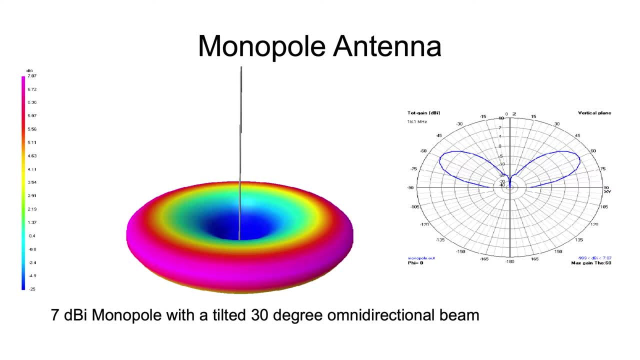 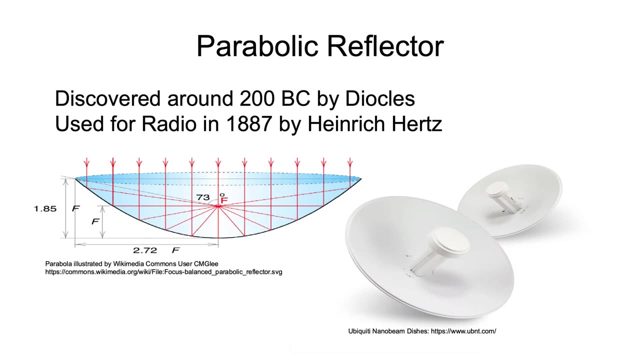 have to be straight, horizontal. It can go up or down. That's what we call tilt in antennas, The parabolic antenna based on a really, really, really old idea. mathematically, if you find a surface for which each integral 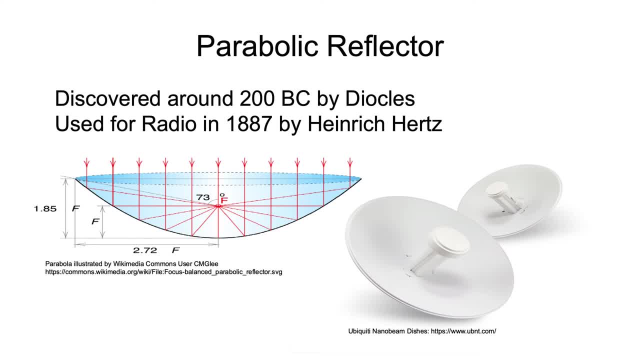 incoming beam is reflected to the same point. imagine you're putting like a dish into the sun, like a mirror dish into the sun, and then that it would concentrate all the sunbeams into one point. That's actually something we're using in solar cookers, solar ovens. 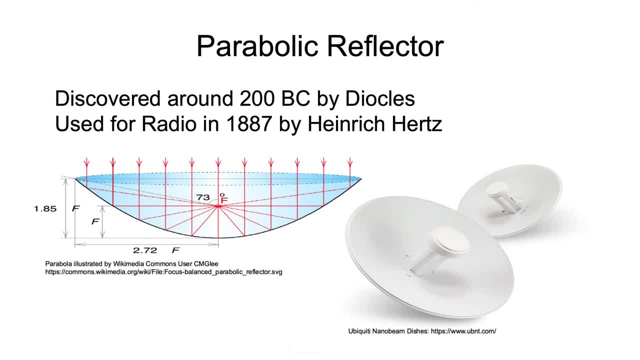 Then that surface that's described as a parable, The mathematical. the finding of this is centuries old- 200 BC. I found as the date for that As a radio reflector also more than 100 years old. that is basically what a dish. 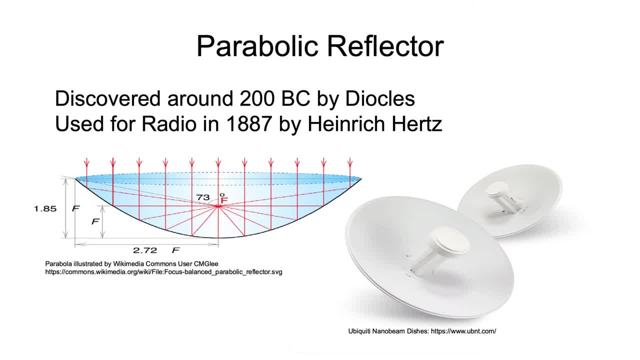 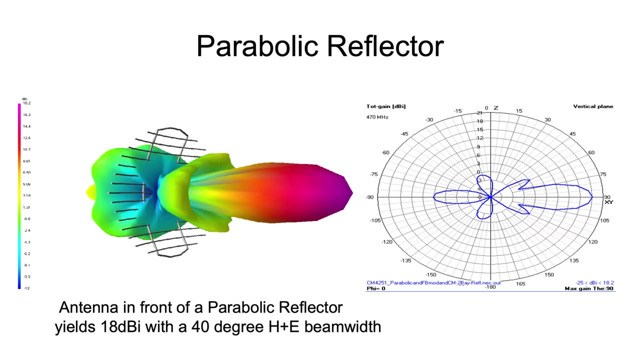 a parable antenna is doing, And you find them in closed types, like those dishes you sometimes also use for TV and radio signals. You find them in grid forms And you can see that the grid is not so much wind resistant When the wind blows. 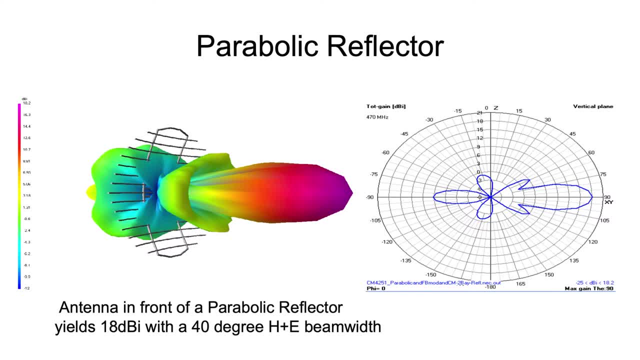 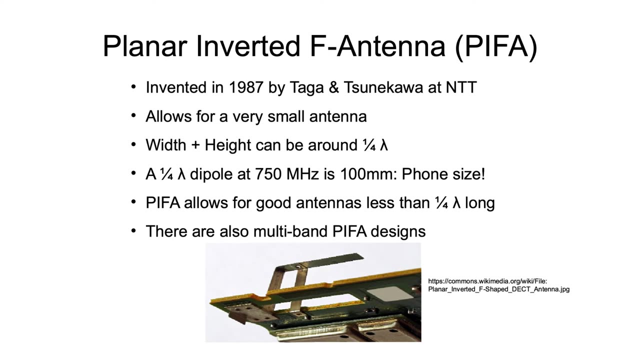 the dishes need to be really, really strong to stand that power of the wind. Grids are better here and they do the same for the electrical, the electromagnetic signal. So that's a grid antenna. Here's another small one that you often find built into mobile phones or IoT devices and stuff. 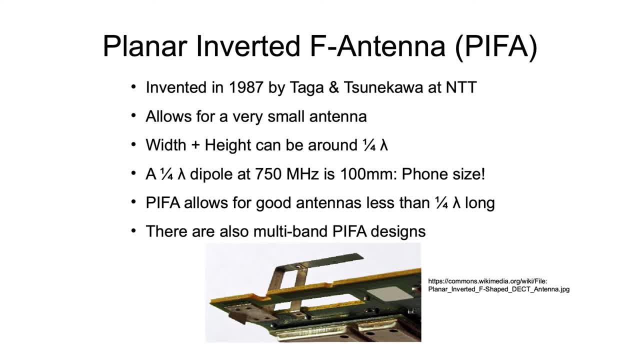 It's a two-dimensional antenna. It's got a plane, but also like an F-shape on top of it, often found, like I said, in embedded boards. and such It's small. You can make it a lot smaller than, say, a quarter wavelength, so you can fit it into these small devices. 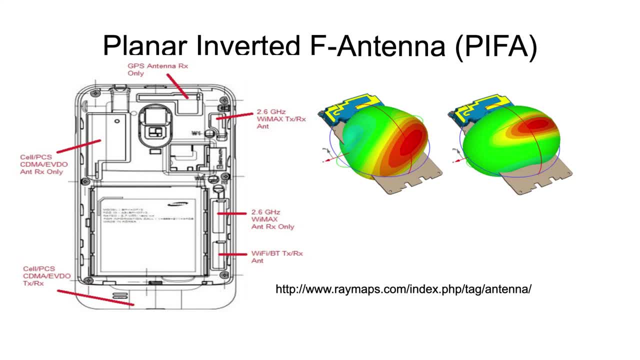 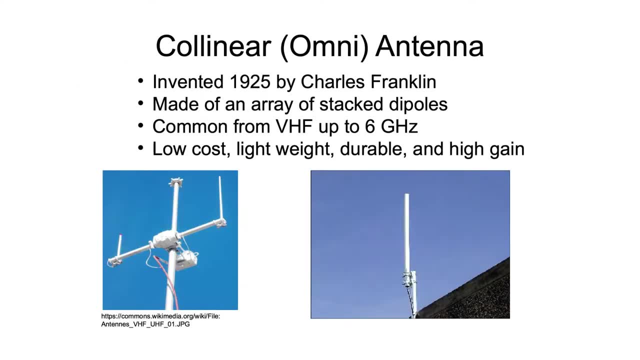 Here's a picture of how these different antennas go into a mobile phone. A collinear antenna is a combination of several pieces of dipole pieces combined together in interchanging polarities, so the effects actually add up. That's why we call them collinear Many. 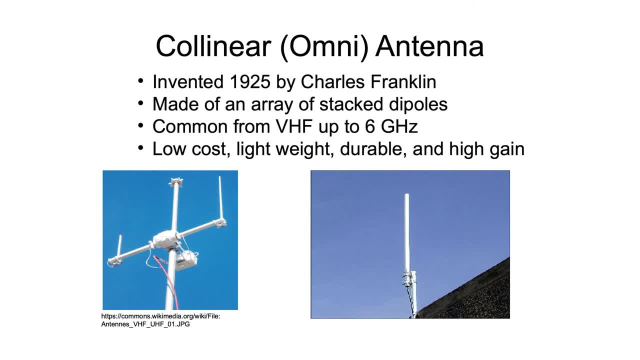 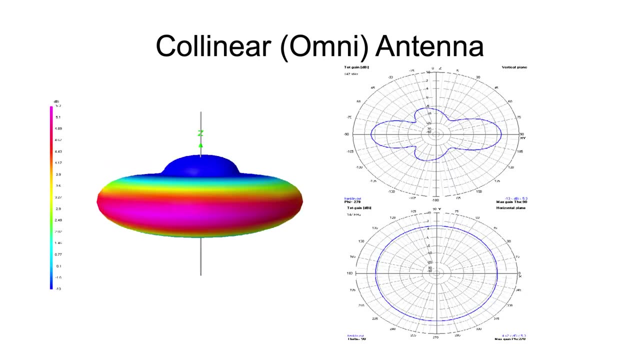 linear elements in one and that gives us an omnidirectional antenna. This is by far the most common type of antenna. We see four omnidirectional uses and from the outside they just look like a stick. basically, This is the radiation pattern for the omni antenna. We've seen it before, Roughly like a 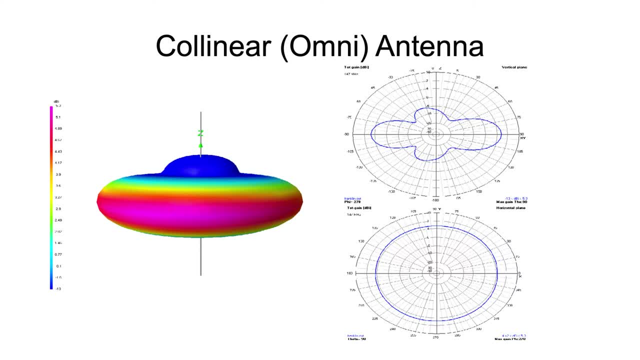 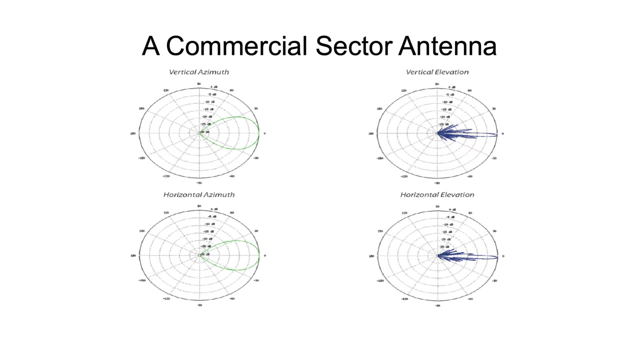 doughnut circle from above and a squeezed something seen from the side directing into two distinct faces. Now let's talk about polar來了. This is our first real camera and you can see that the previous camera had a wide beam that has the ability to draw at the end of a line. We saw two cameras doing this: A long beam on one side and a wide beam on the other side. If it's a long, then we speak of a tilt. This is what commercial sector antennas look like. They're a combination of several patches inside, So they're actually a long square and the resulting pattern is a wide beam into one distinct direction. wide beam into one distinct direction and two different directions. 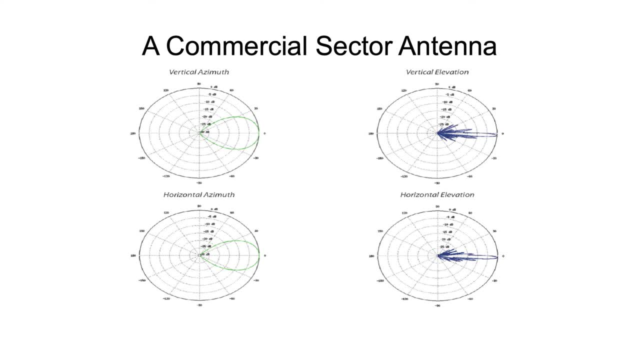 can mean anything from 30 degrees, 44, 45, 60 degrees, something like that. this would be the radiation pattern for a uh such a sector antenna wide, seen from the in the horizontal plane here and looking at the elevation and for the two polarities, you see a relatively sharp, a relatively thin. 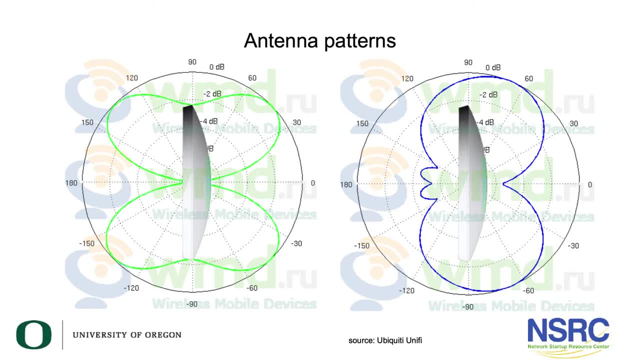 beam width. here's another pattern, for many of you might have seen the sort of patch on the wall type of antenna, often with the axis point integrated into it. this would be the radiation patterns for such a type antenna. note that it's actually not strongest towards the center but the 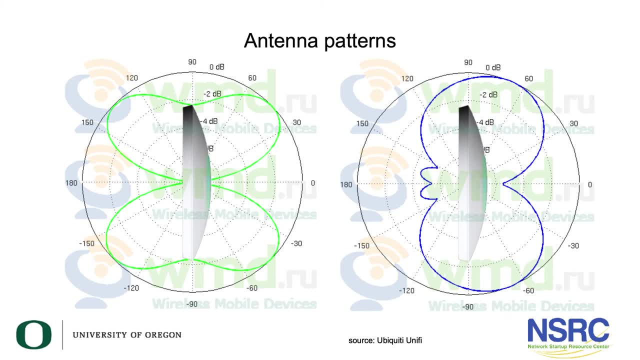 directions of strongest signal is kind of off center around it, so don't direct it directly at where you want to go it. it spreads out the signal. it's meant to ideally sit on the ceiling, perhaps on a wall, but its main usage would be overhead on a ceiling. 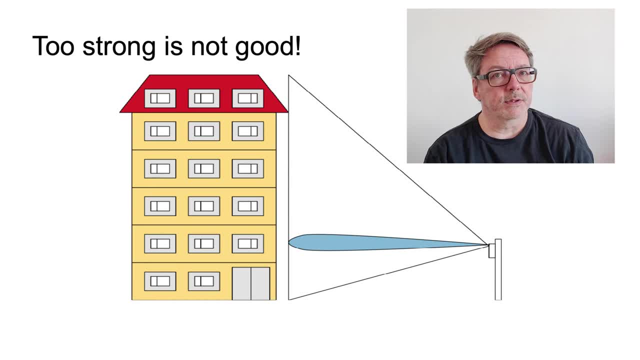 a little comment on choice of antennas. don't always go for the strongest. um. here's an example of we've chosen a very, very serious antenna. the main utility for the majority of us is that they are still on the ceiling and that they should be in a one-way position and the antenna's growth. you can see in this picture that the antenna's growth is in a vertical line, and so the way that we're doing this is going to be on the ceiling instead of on the wall, and the antenna's long and then the antenna's length is going to be on the ceiling, and that's what a lot of people 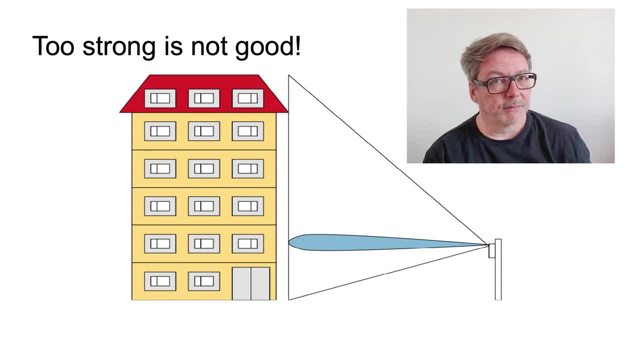 we are looking at is often the use of antennas that are not flat and they should all be in the middle of the very, very strong directional antenna. but if we want to hit all of this building here, we actually don't want such a strong directional antenna, we want a spread. 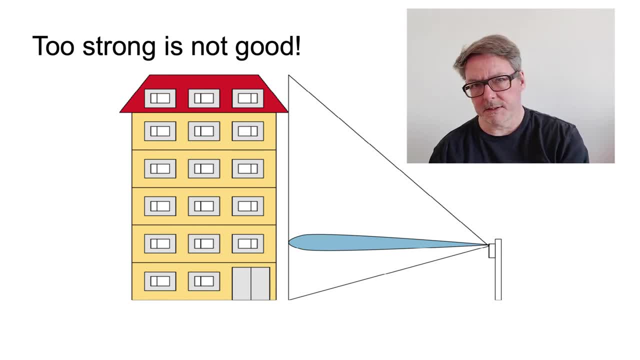 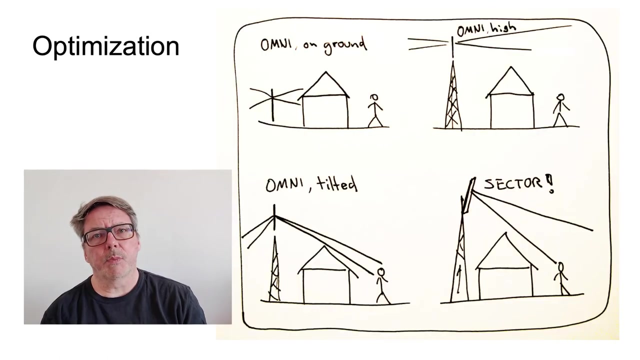 we want a wider beam width. probably, looking at this picture, we want 60 to 90 degrees, not a thin line. we want to have a relatively weak directional behavior in order to hit all the flaws of this building. here's one more little um. look at how we're choosing antennas. 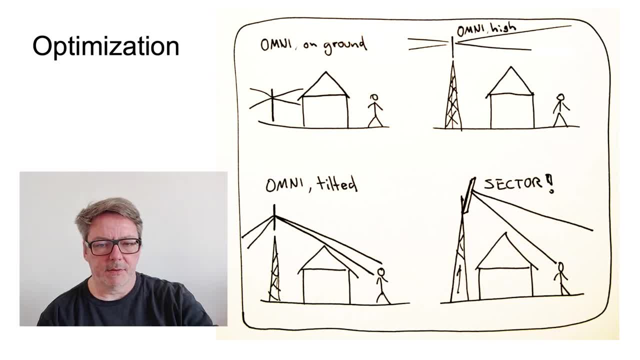 let's say we have this case. we have a person behind the house. this is who we want to reach. we have an omni antenna behind that building. obviously, that's not a very good solution. our first reaction is: well, bring it up, bring it onto a tower. um, that's somewhat better. however, now we have the problem that 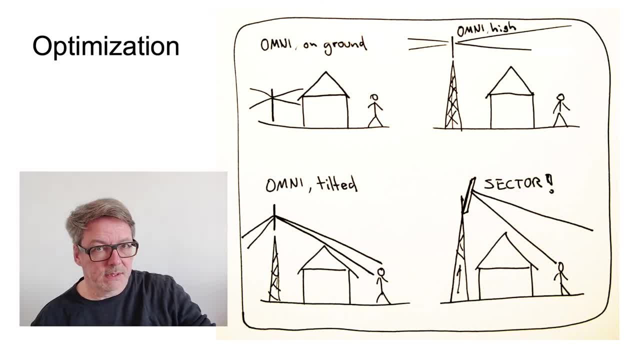 we're missing the receiving side. we're missing the user. our next reaction to that is we'll use an omnidirectional with a tilt down. that's better. however, most of our power is still going into directions where we don't need it at all, so our next improvement would be to use a sector. 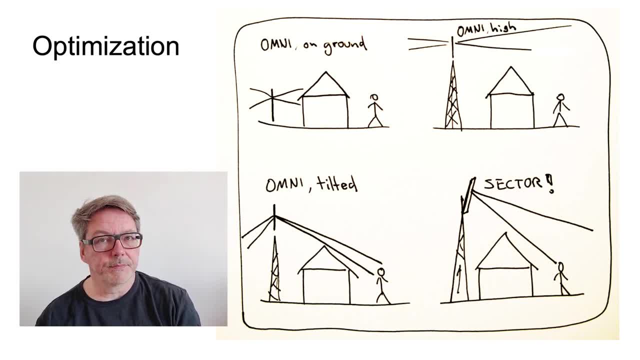 antenna instead of the tilted omni. make such drawings when you're planning antennas. they're very, very useful. just pen and paper, try to. you need to know where your users are, where you are, the receiving end of your signal. you need to know where you want to put your antenna.